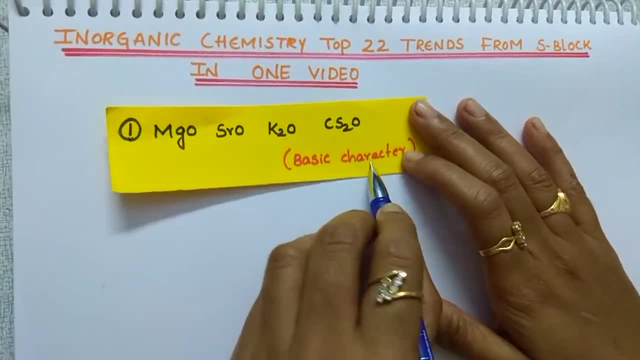 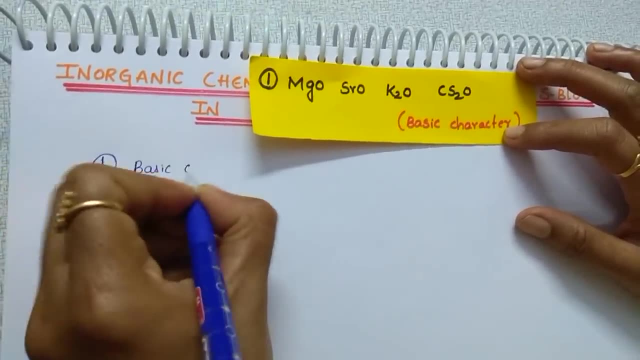 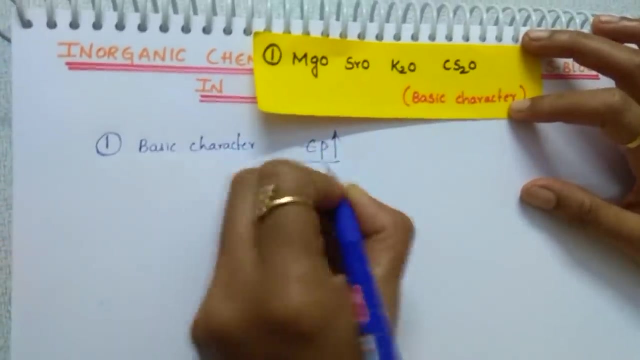 am taking an increasing order which is having more basic character. So more basic character. how you have to solve students. Basic character is: more is a electropositive character, more is the basic nature. More is a electropositive character, more will be the basic nature. 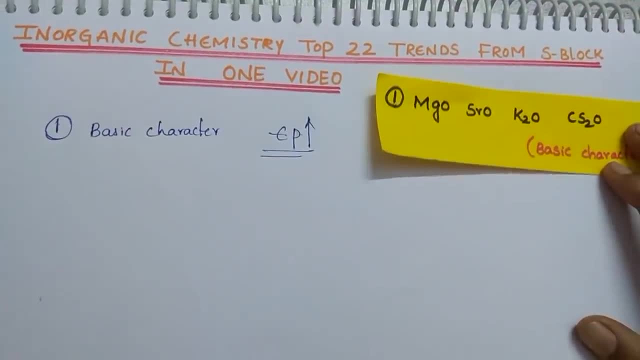 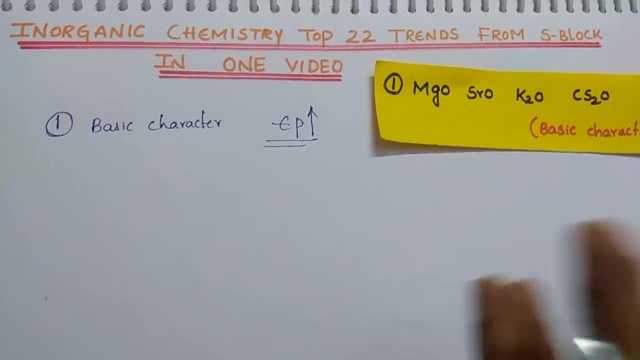 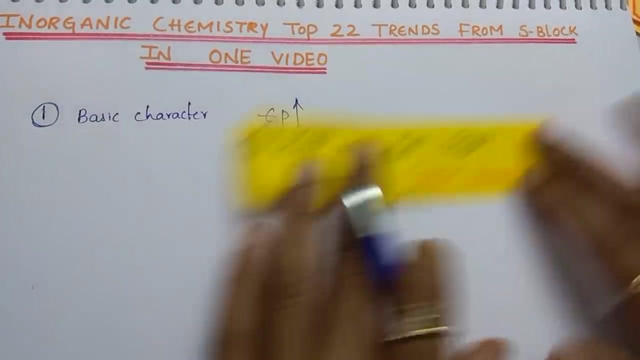 What is the point here? Electropositive nature of the metal is more so that basic character of that oxide is more How you will find the electropositive character? completely based upon metallic nature. Size increases or automatically electropositive character increases. Then what? 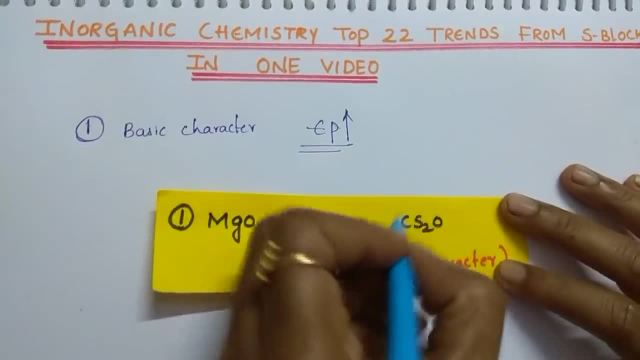 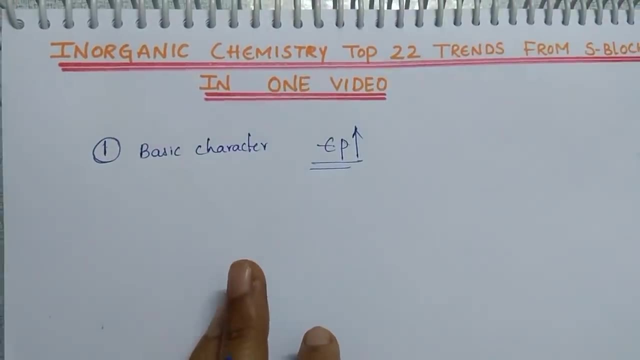 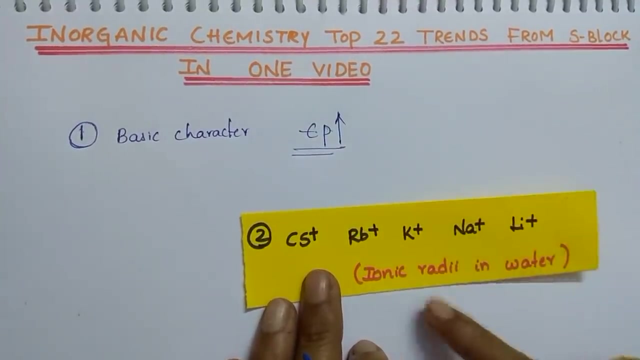 is the trend here. So what is the correct trend? CS2O is having more than K2O, then SRO, MGO. Let us see the next question: Cesium ion, rubidium ion, potassium ion, sodium ion and lithium ion. you have to find. 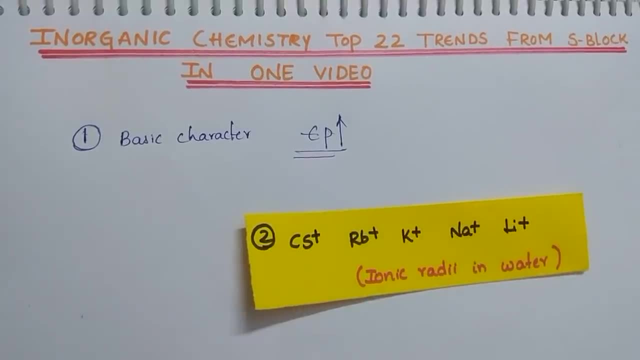 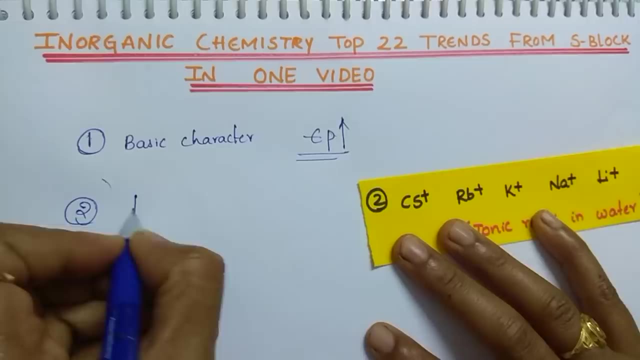 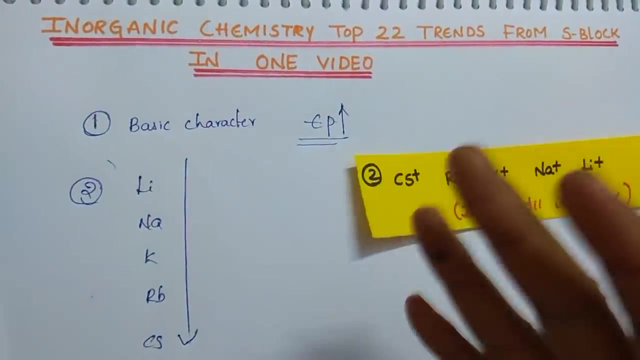 the ionic radii in water. which is having first find, which is having smaller radii and which is having larger radii Top to bottom. what happens to the size? students tell me Lithium, sodium, potassium, rubidium, cesium, top to bottom size of the atom increases. So obviously. 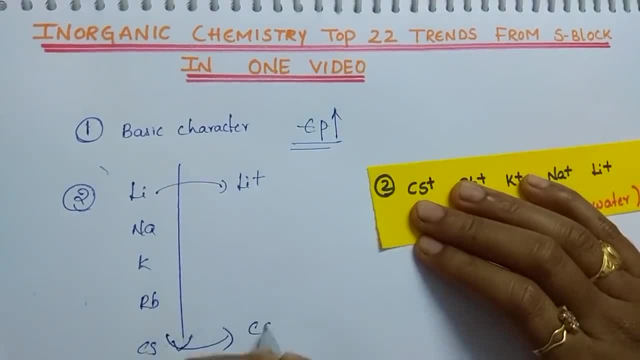 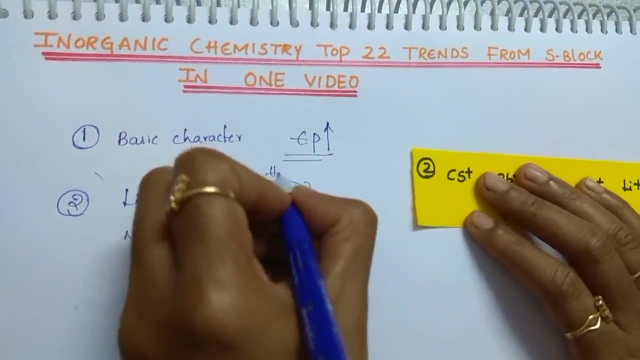 lithium ion will be smaller in size and cesium ion will be smaller in size. So you have to find the size. Cesium ion will be larger in size, This is small, this is smaller, this is larger. But when you put this in water, the smaller lithium atom holds more number. of water molecules. This is in one water molecule- like this, all are water molecules- more number of water molecules it holds. Whenever it holds, more number of water molecule, the size of lithium ion in water will be more, Whereas cesium ion is having a larger size than the. 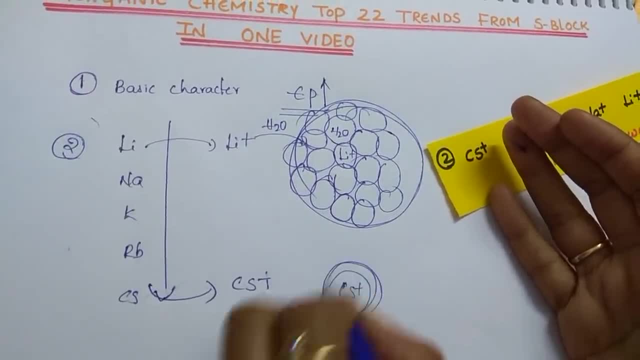 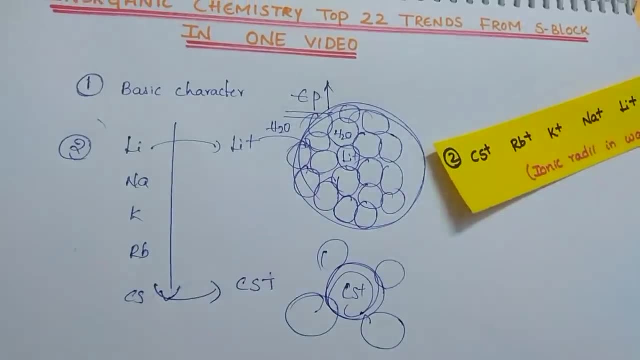 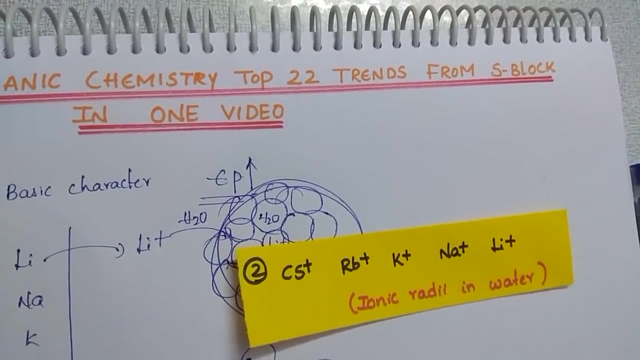 insane: No size and it cannot hold more number of water molecule. like lithium, It holds very less number of water molecule. So that size of cesium ion in water is LESS. Now what is the correct increasing order? which is having increasing, which is having a larger ion size? 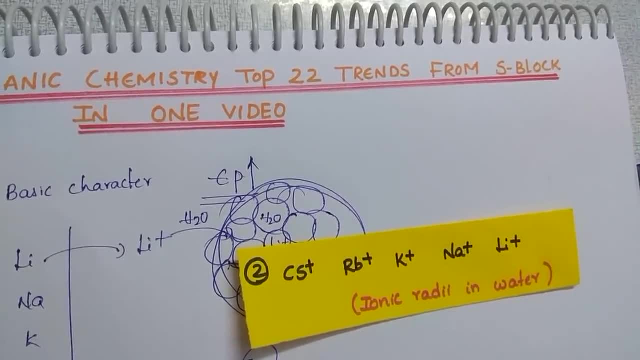 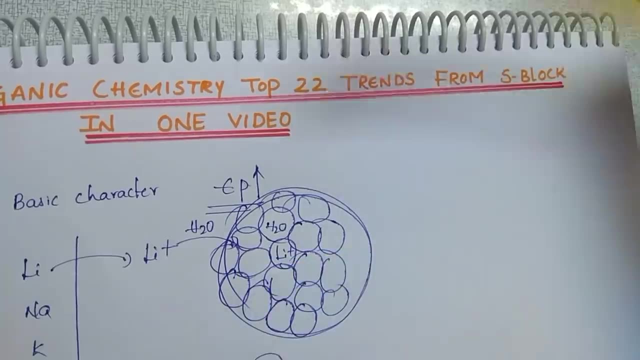 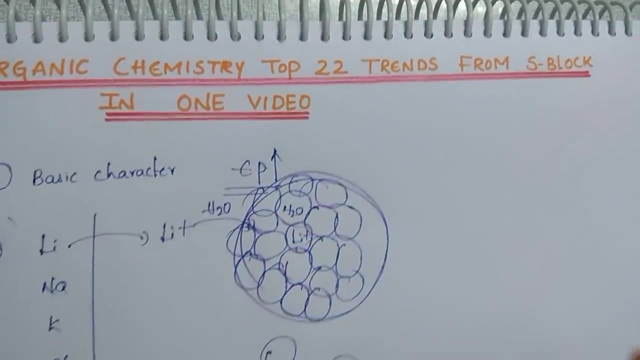 in water. Lithium is having larger size in water. Whenever it is having a larger size, tell me which is my size. Other小 beginner can understand which is my size or which is my me, which is having the ability to, which will move faster, either lithium ion in water moves faster. 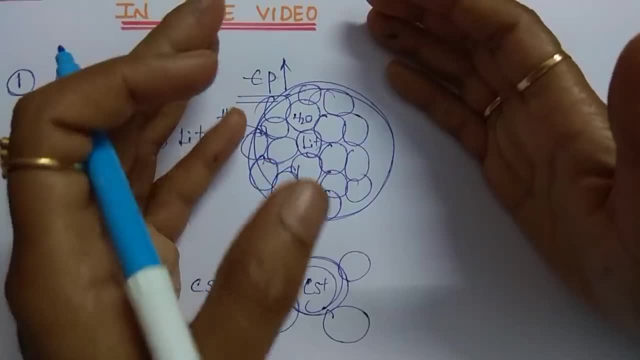 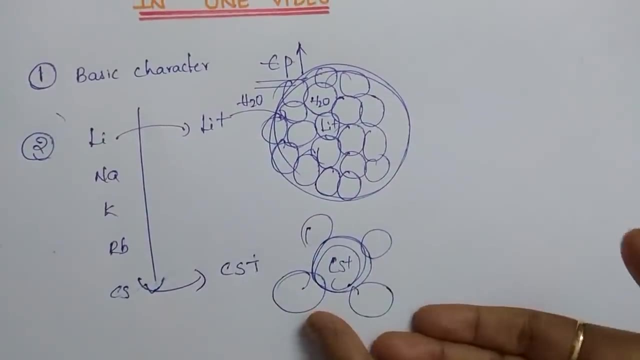 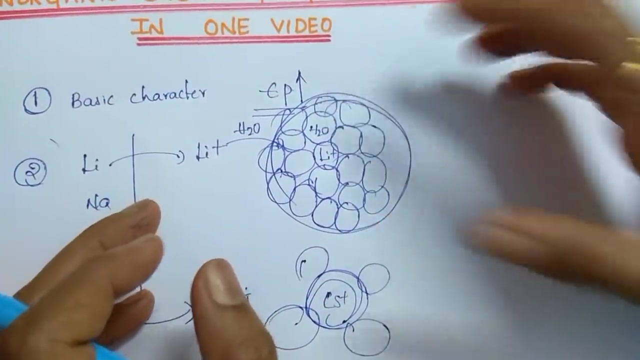 or cesium ion in water moves faster. 100 kg person, 50 kg person- running competition, who will win? obviously 50 kg, 100 kg, they run slowly, for example example. okay, so here lithium ion in water is having larger size, so it moves slowly. now tell me which is having molar conductivity in water. 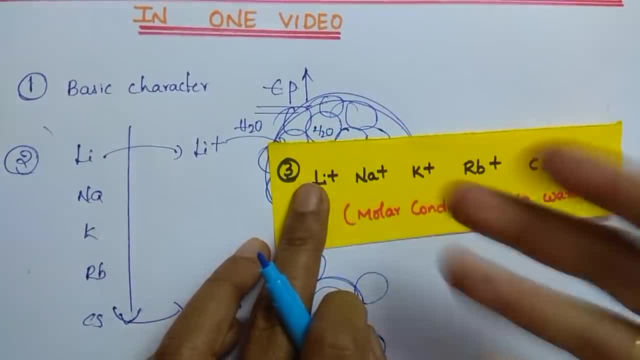 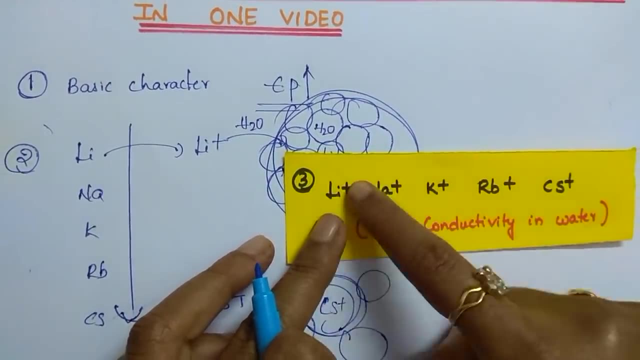 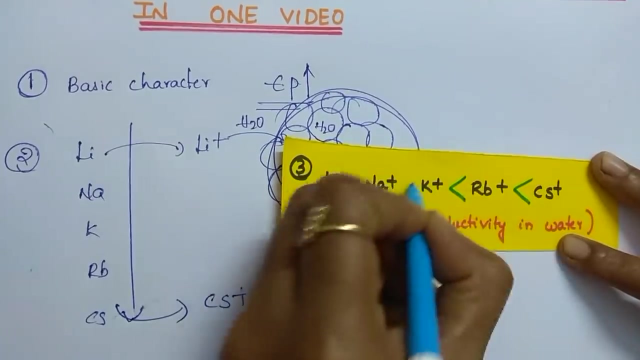 smaller is the size of an atom ion, so that it moves faster. but in case of this ions in water, it is having more hydration energy. it is hydrated more so that it moves slowly. cesium ion is hydrated less, so it moves faster. right, next question: lithium sodium. 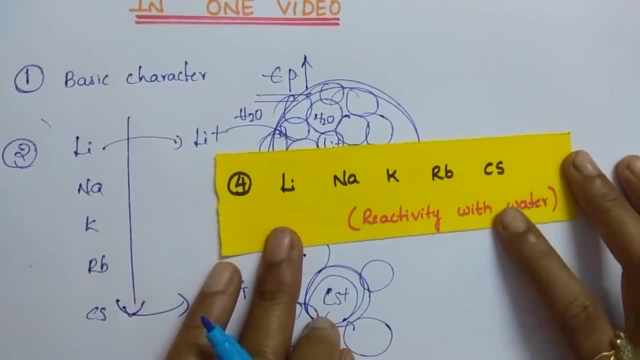 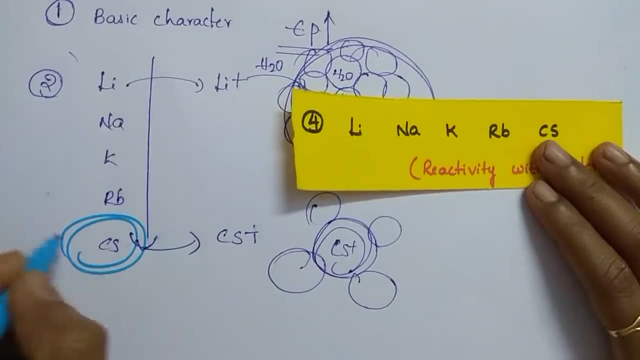 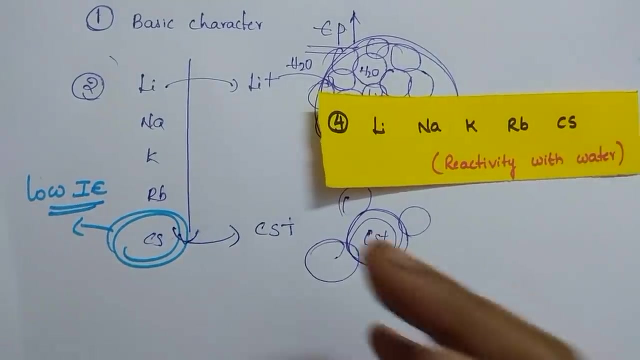 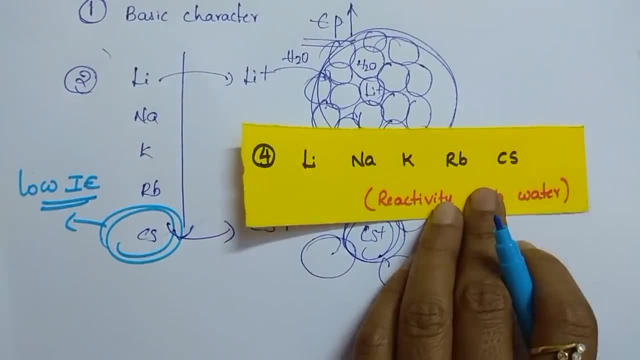 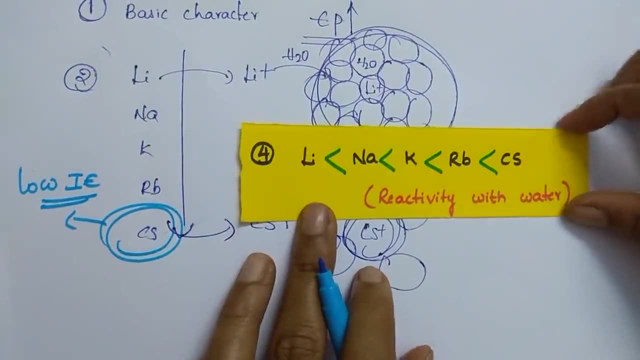 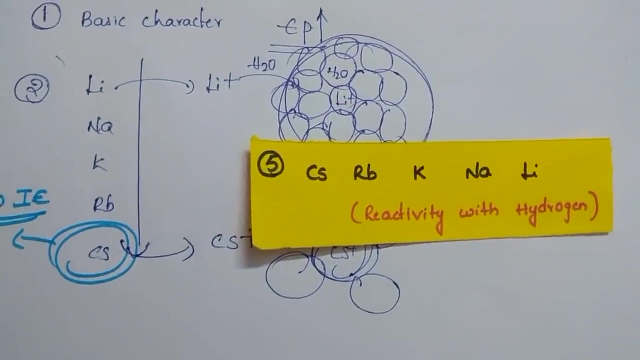 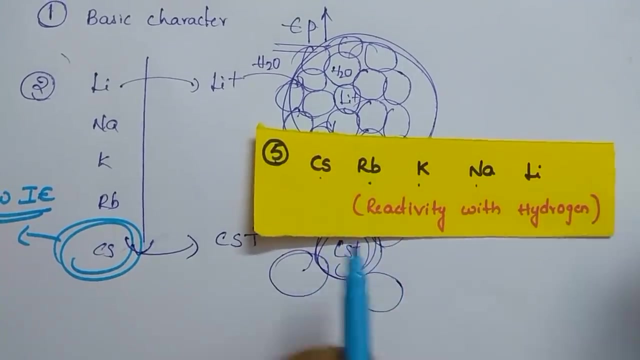 cesium ion is having low ionization energy, more metallic nature and it reacts with water faster. so this is the correct order. got it students clear: more trends: you are going to learn see how. how difficulty trends. also, you are going to learn in an easier way: lithium sodium, potassium, rubidium, cesium, which one reacts faster with hydrogen lithium ion. 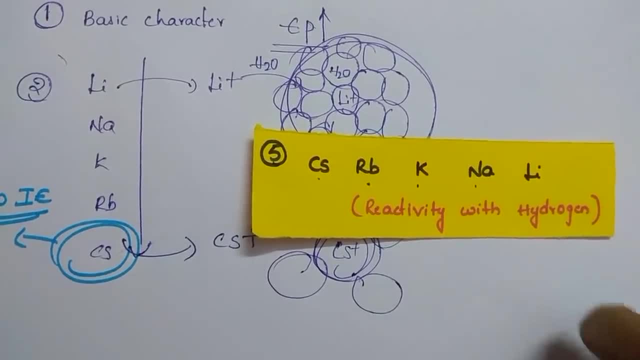 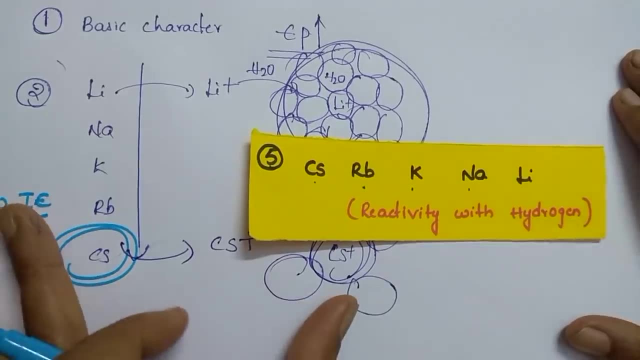 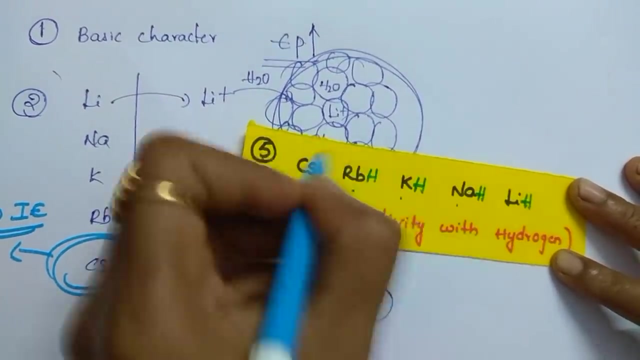 lithium atom forms lithium ion, whereas hydrogen reacts with it, with these alkali metals and forms lithium hydrides, means alkali metal hydrides they form. it forms lithium hydride. it form sodium hydride, potassium hydride, rubidium hydride and cesium hydride in 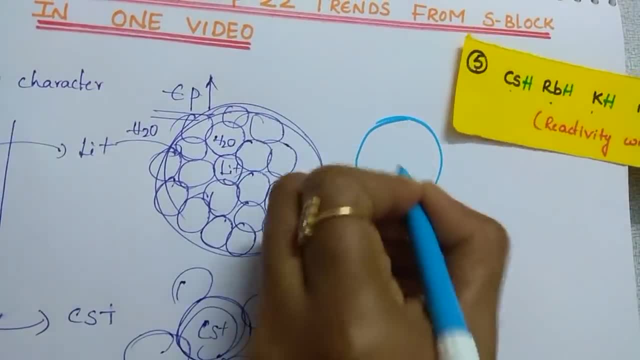 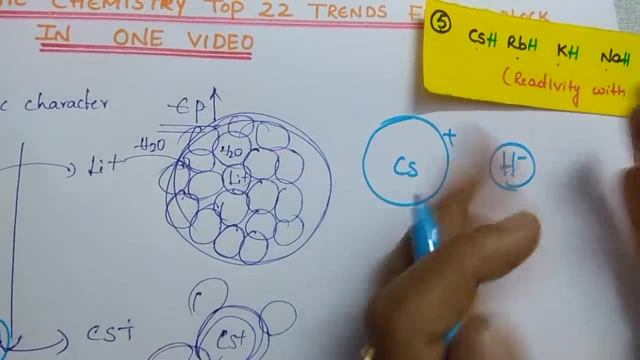 case of cesium hydride, what happens is: this is the cesium ion and it is a hydrogen ion. then both: it is a larger ion, it is a smaller ion. the bond between the two is weak. so it is. we can say it is a less stable hydride, it is a stable hydrogen ion. 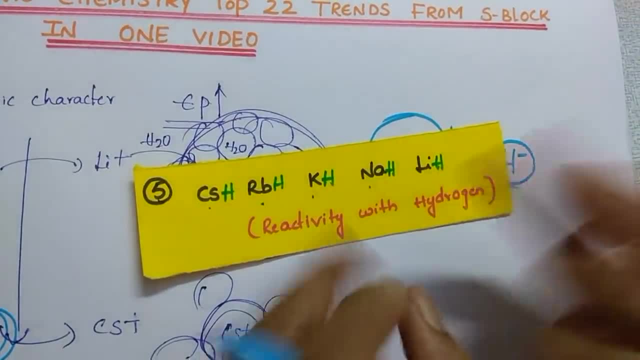 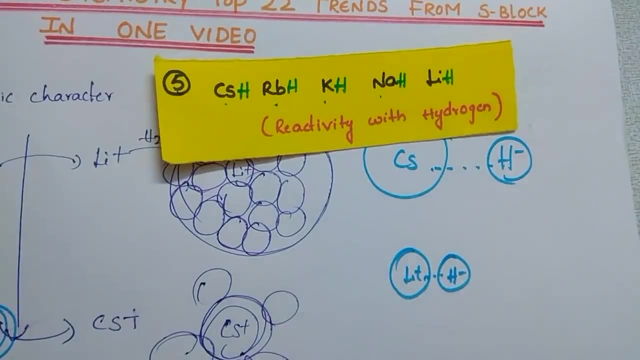 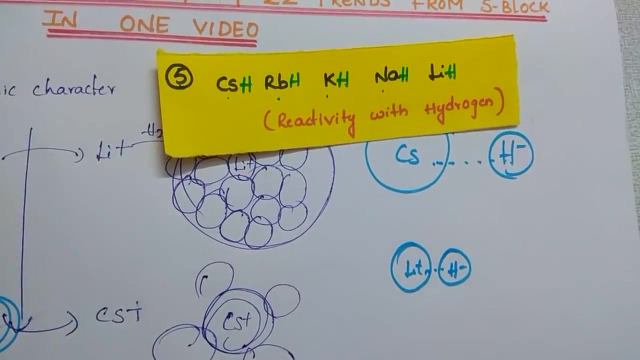 this is a more stable hydride to because the lithium atom ion is a smaller ion and hydride ion also smaller, so that it holds tightly. lattice energy is more in this case, so that its stability also its stability is more to get that stability which, if you see lithium and cesium lithium, reacts. 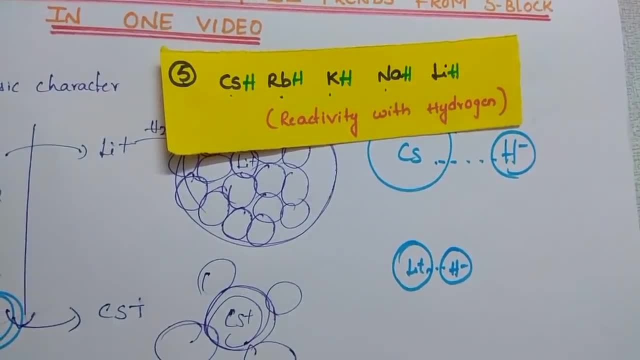 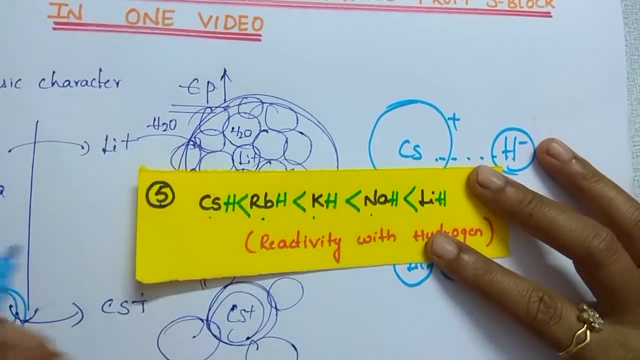 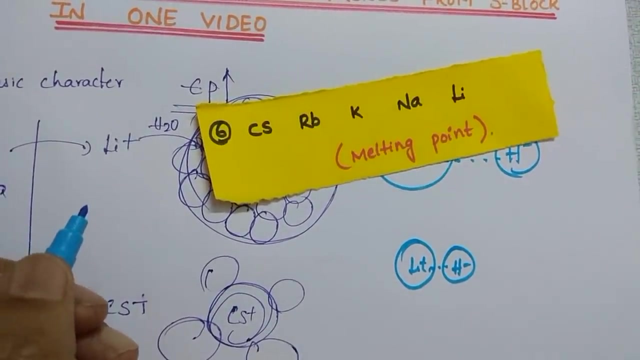 with hydrogen faster and it forms the stable hydride. now tell me what is the correct trend, students. lithium hydride, sodium hydride, potassium hydride, rubidium hydride and cesium hydride. tell me the melting and boiling points of alkali metals: lithium, sodium, potassium, rubidium, cesium. 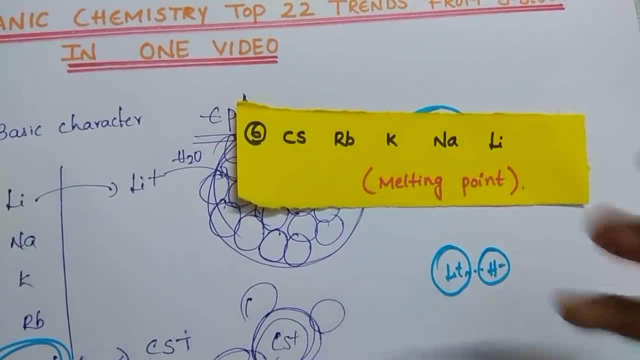 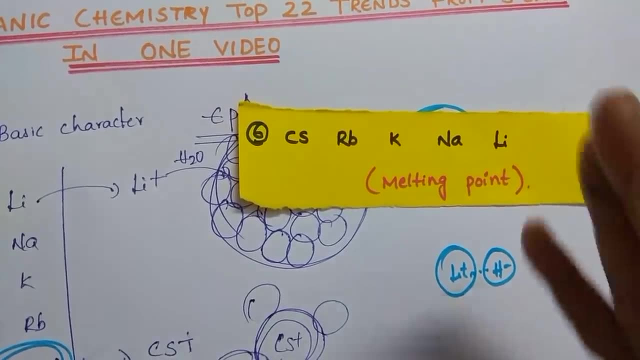 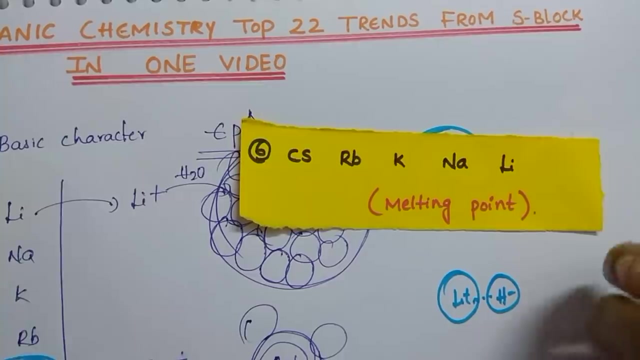 what do you mean by melting point? the temperature at which solid converts into liquid. we call it as what melting point. what is that temperature at which solid converts into liquid. we call it as melting point right and melting point we? it depends upon number of electrons in valence shell. 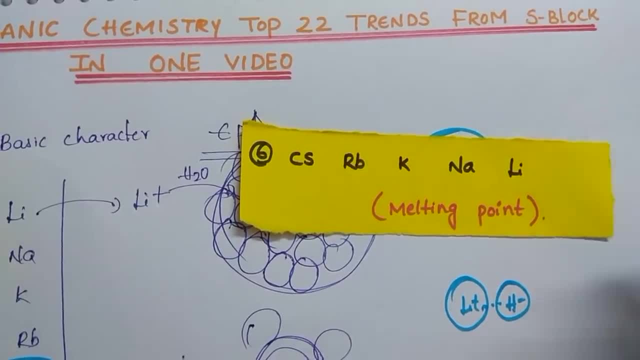 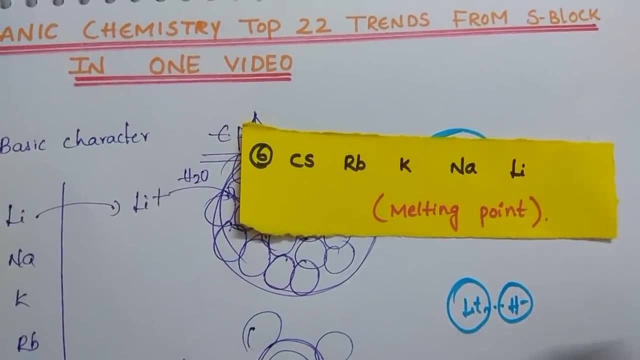 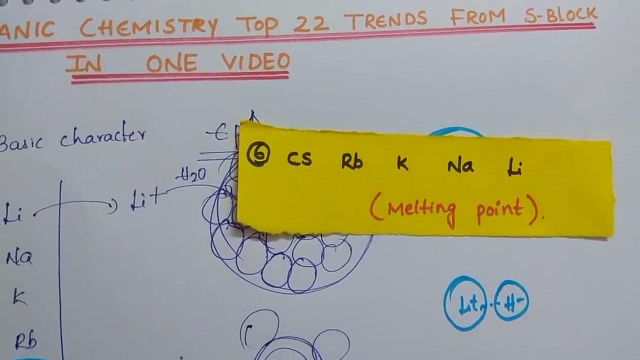 because more is the number of electrons in the valence shell, so that force of attraction between the atoms are more. whenever force of attractions are more, it's stronger is a metallic bond, so that it needs a higher temperature to break those bonds. but in case of alkali and alkaline earth, 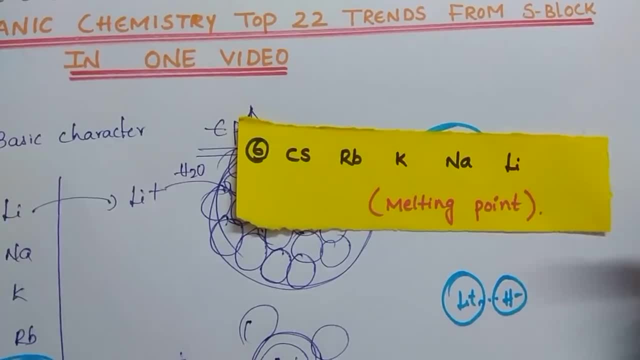 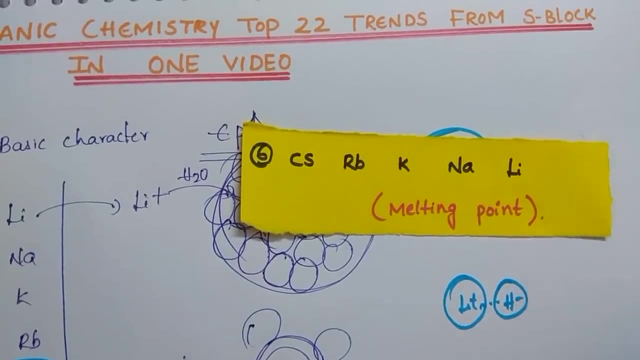 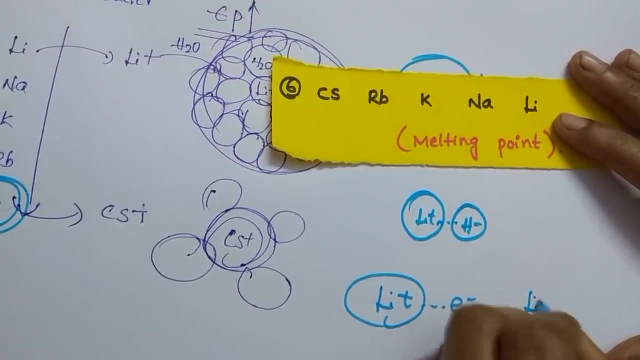 metals. less number of electrons there, usually alkali, only one electron in valence shell. they they show weak force of attraction between the atoms whenever they have weak forces of attractions between the atoms like this, due to only one electron, the force of attractions. we say these force of attractions as cohesive forces. 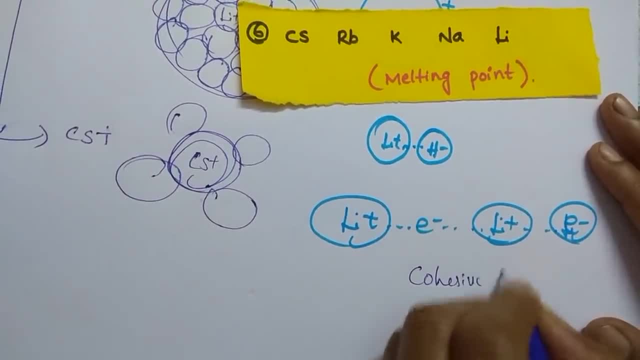 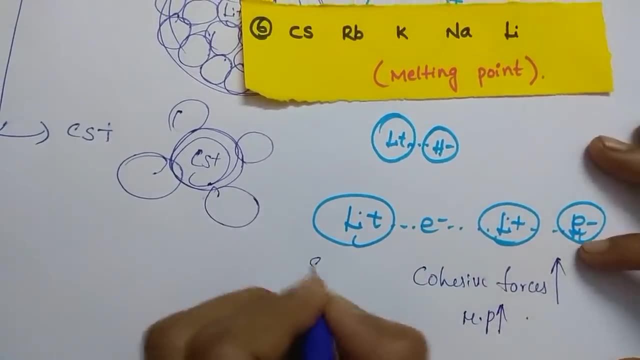 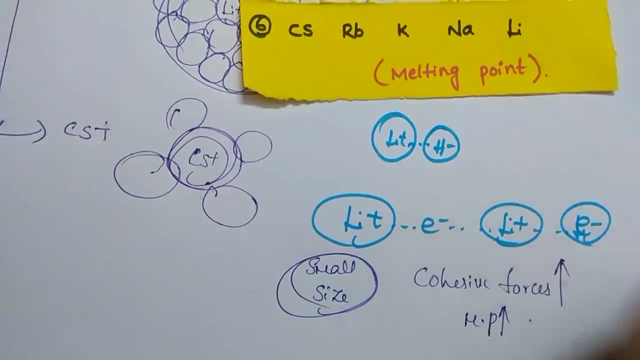 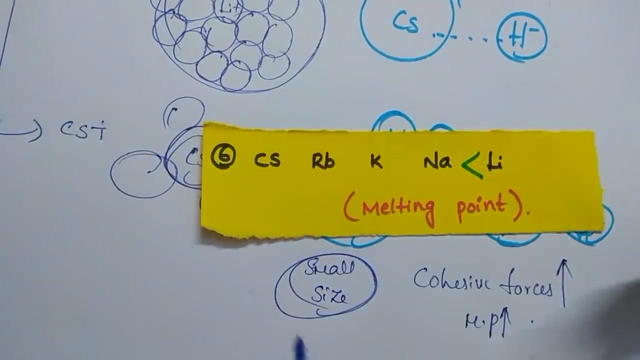 what is the students? cohesive forces, cohesive forces. if cohesive forces are more, melting and boiling points are more, which one shows the cohesive forces. small sized atom shows more cohesive forces. small size means more cohesive forces, more forces of attractions. then melting point will be more. lithium is having a smaller size so that it shows more cohesive forces, stronger cohesive forces. 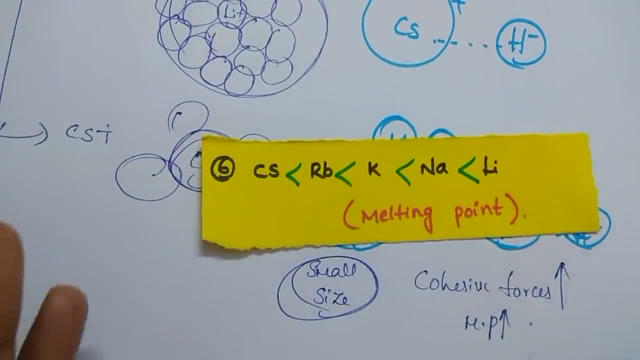 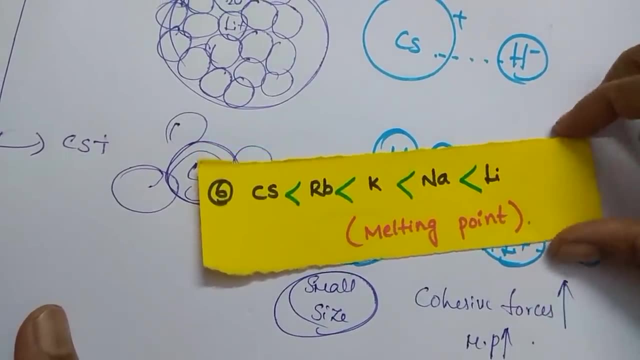 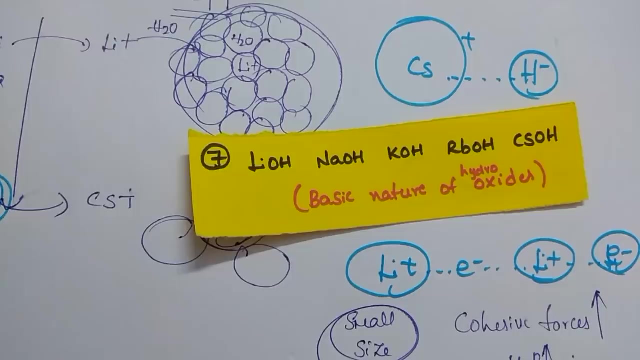 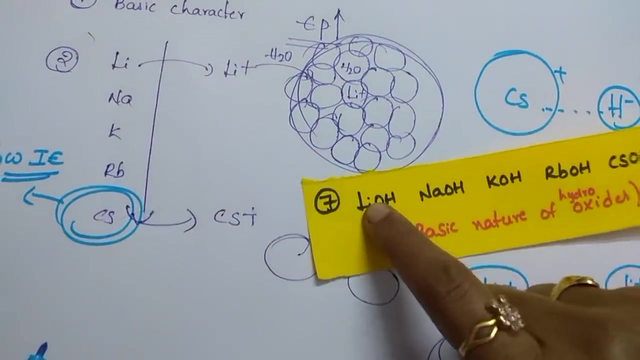 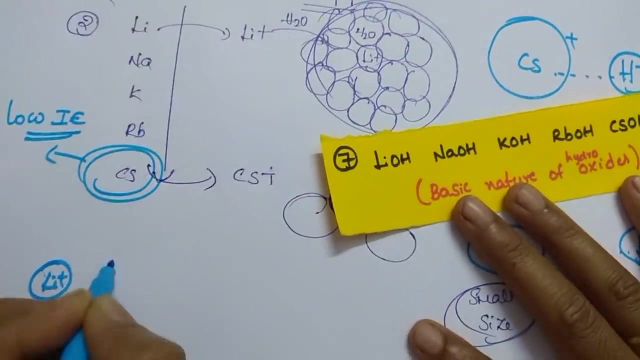 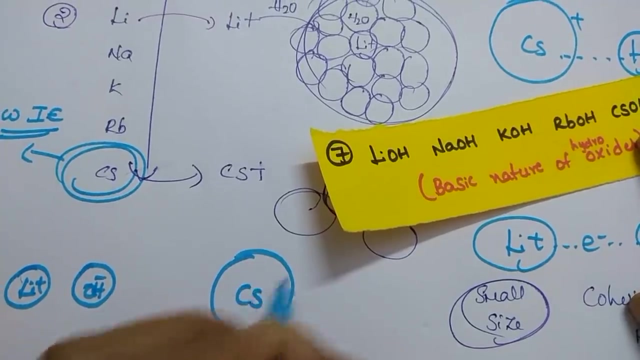 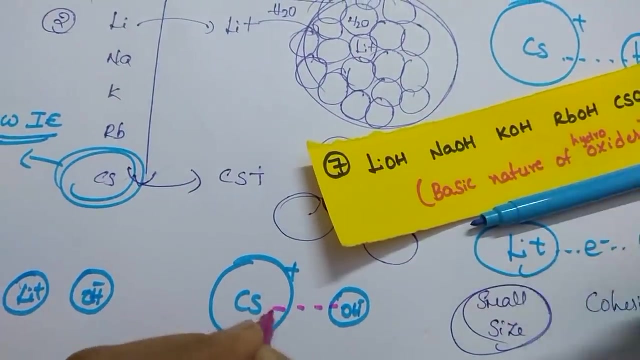 when compared to cesium, and usually they have alkali metals, have low melting points because of the presence of single valence electron, only one valence electron, our oh minus ion, Which bond is a weak bond. This is a weak bond due to larger size of cesium and smaller 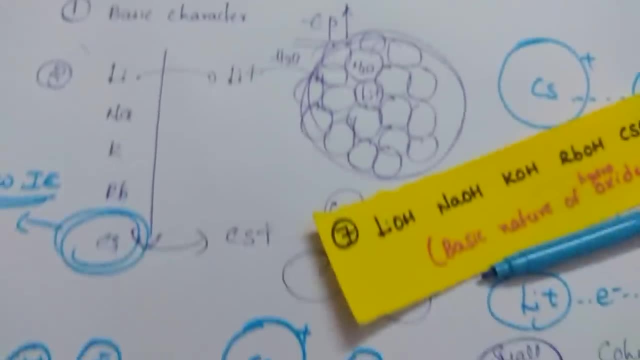 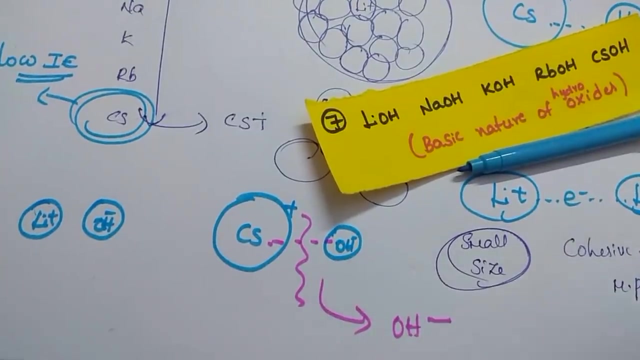 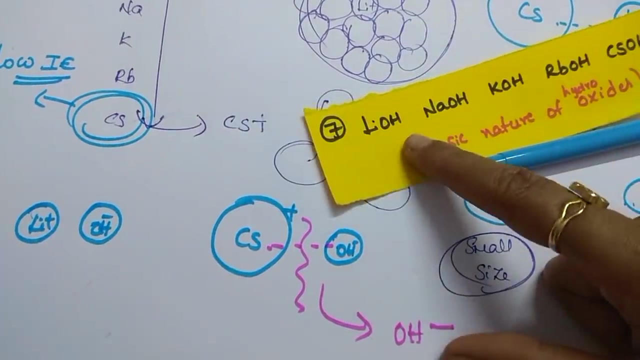 size of OH minus ion. it is a weak bond. Whenever it is a weak bond, it this bond breaks easily and it gives OH minus ion easily. Whenever it gives OH minus ion easily, we say it is more having more basic character: lithium, hydroxide sodium, hydroxide potassium, hydroxide rubidium, hydroxide cesium. 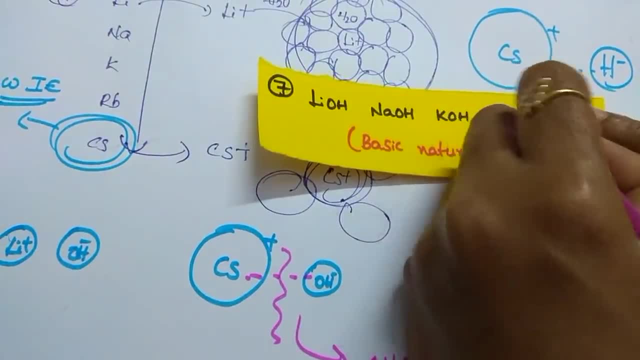 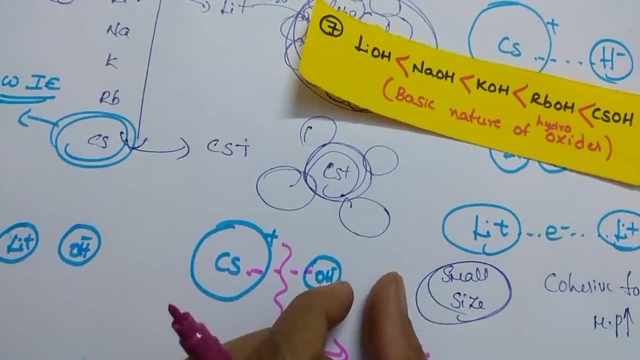 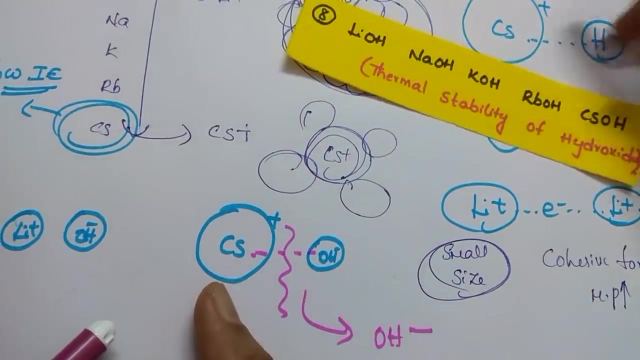 hydroxide which is having more basic character. Cesium hydroxide is having more basic character. why? Due to the larger size of cation and smaller size of anion, the bond breaks easily and gives OH minus ions easily. Tell me the thermal stability of hydroxide. Here I am going to tell you a small. 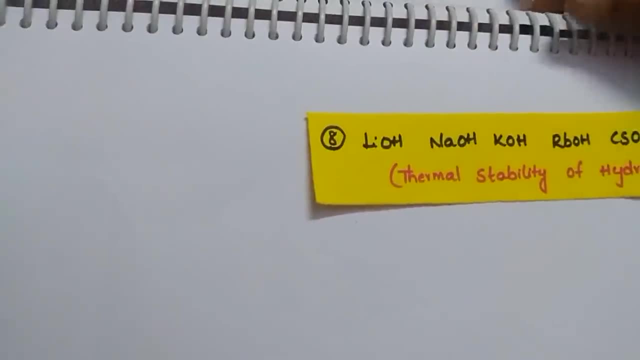 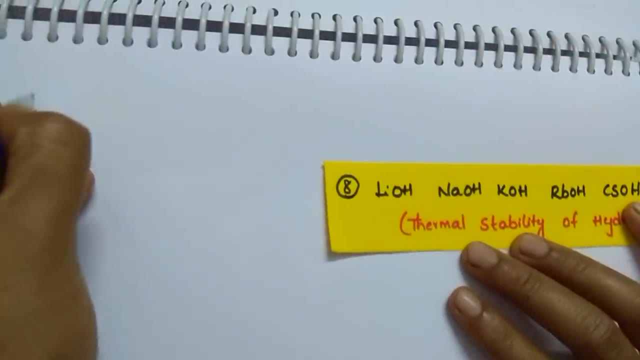 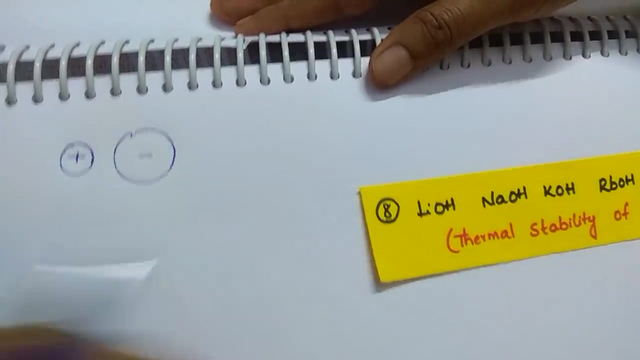 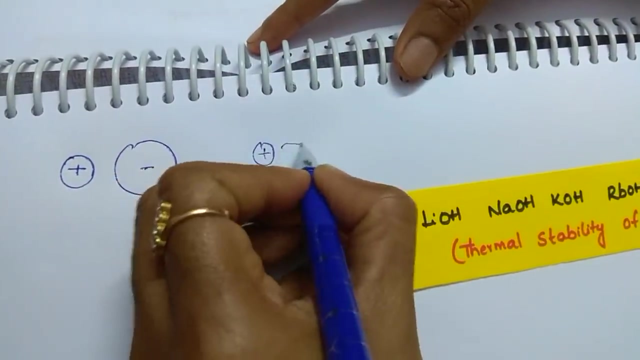 trick. this is from Fersenstuhl. If you understand this trick, you can solve the next coming questions very easily. See, whenever size of cation is smaller and size of anion is larger, so that cation will attract the electron cloud of the anion Slowly. whenever cation attracts the electron cloud of anion, 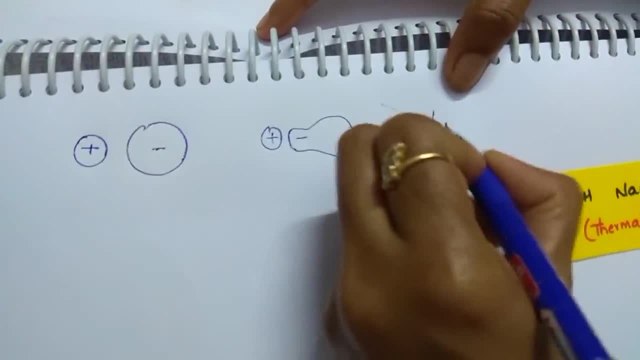 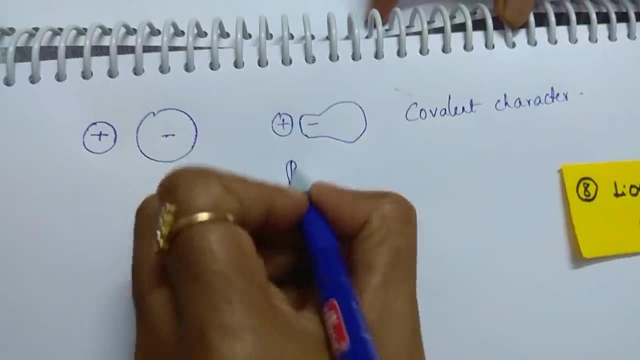 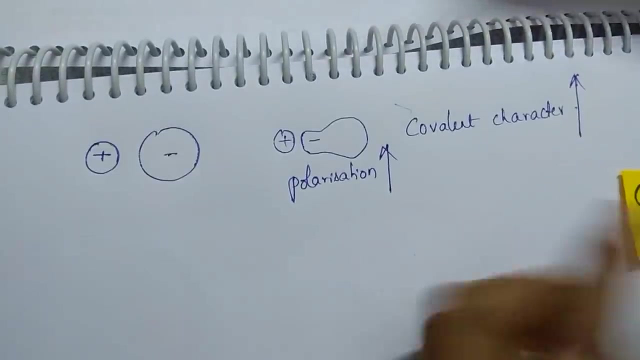 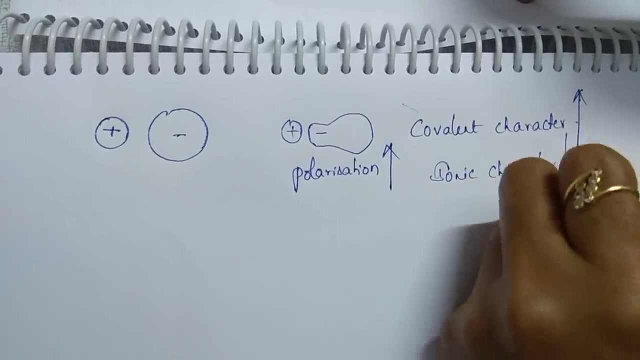 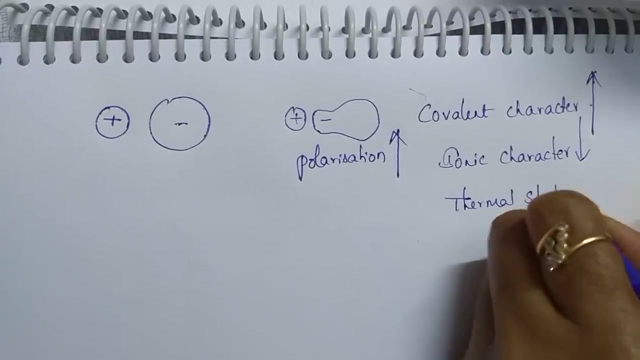 towards itself. covalent character increases When covalent character increases. students tell me: polarization When polarization increases. covalent character increases When covalent character increases. ionic character decreases When ionic character decreases. what happens to thermal stability? is thermal stability decreases When thermal stability decreases? you say melting? 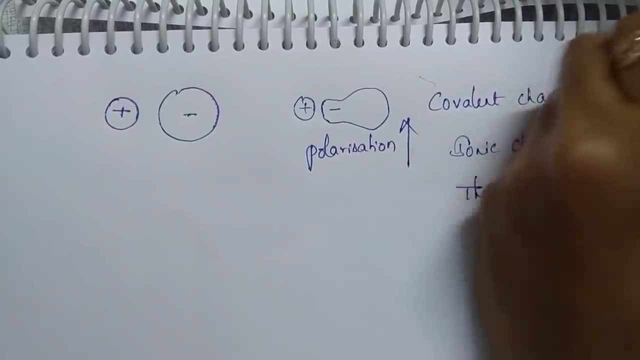 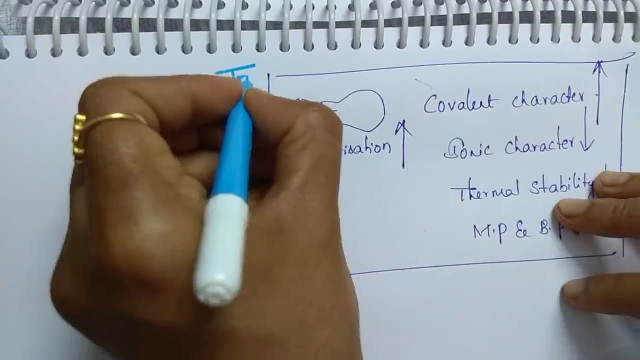 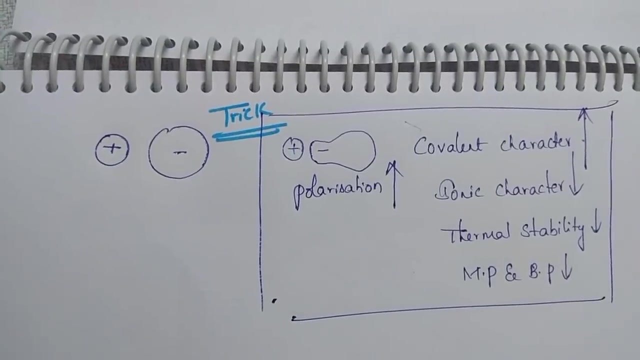 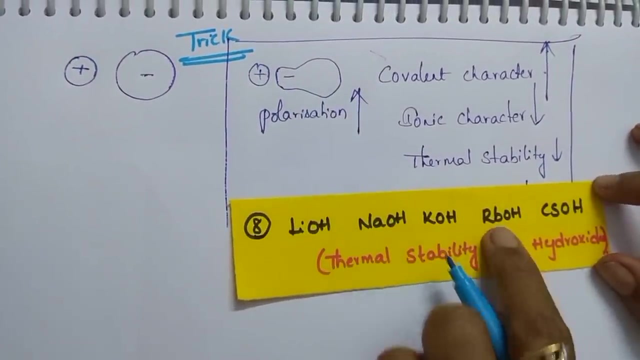 and boiling points also decrease. this is the trick. just once, go through this trick, note down these points and solve the coming questions. I am sure you will be very happy with these kind of questions without any confusions. you will solve lithium hydroxide, sodium hydroxide, potassium, rubidium and cesium. 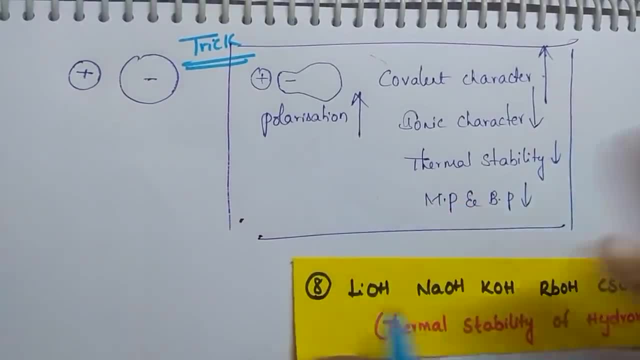 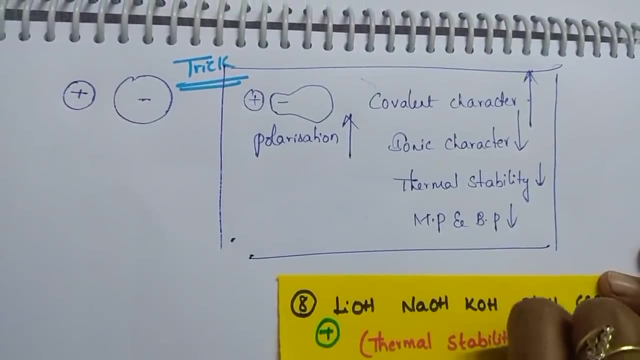 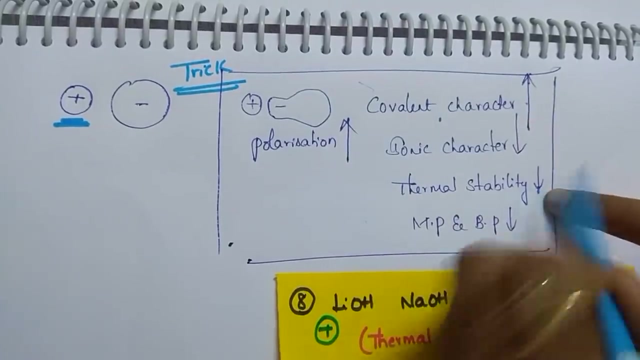 just now I told you lithium ion is smaller size. anions are same, so don't worry of that. this is a smaller cation. this is a larger cation. small cation means small cation is having more covalent character and less thermal stability, so it is less thermal stability. 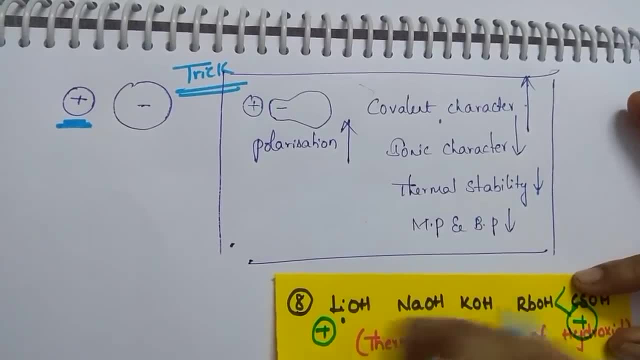 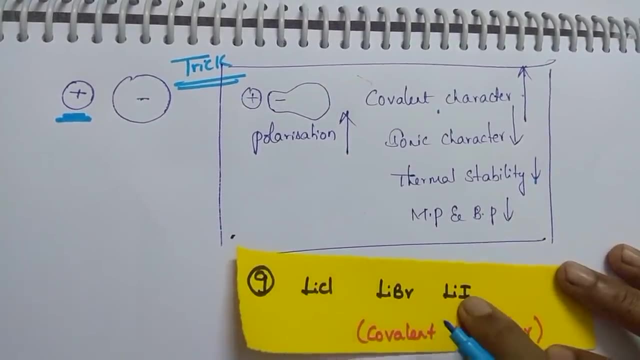 obviously larger cation will have more thermal stability. that's it. that's it. see the next question: lithium chloride, lithium bromide, lithium iodide. find the covalent character which one will be having more covalent character, small cation. 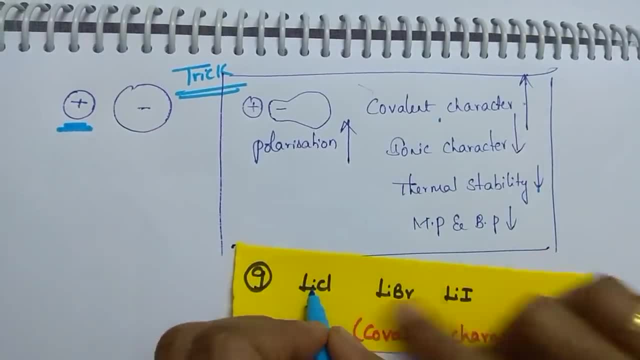 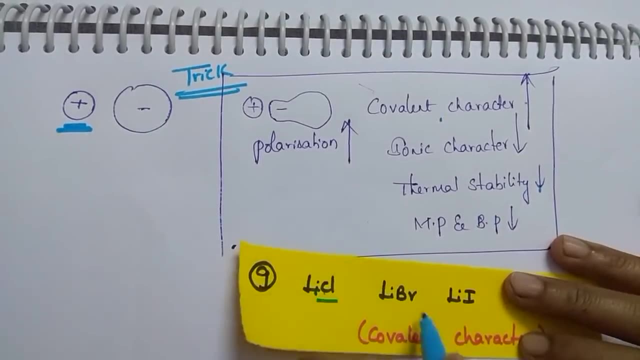 of cation and large size of anion. this is lithium, lithium, lithium, same. no need to worry of cation which is having a larger size of anion. lithium, bromine, iodine, iodide chloridine. 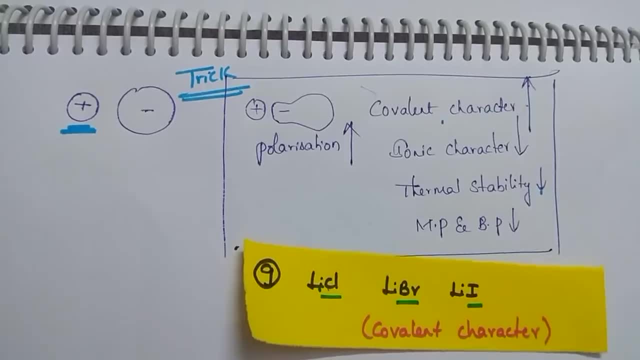 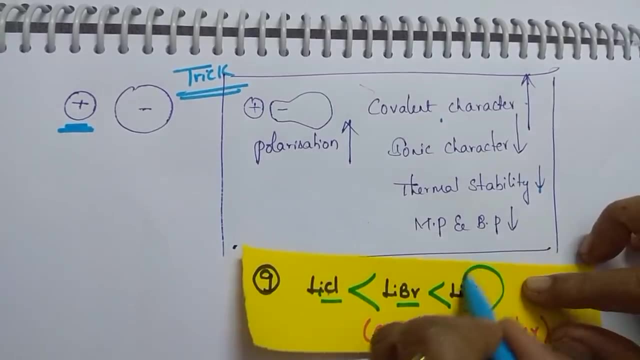 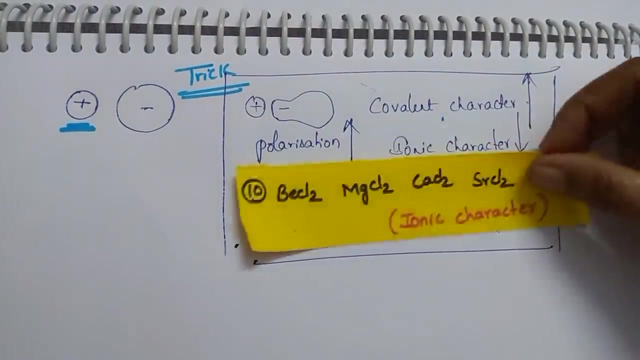 bromidine iodidine top to bottom. what happens to the size of halogens increases. so lithium iodide is having more covalent character than lithium bromide. lithium chloride- larger size, little smaller, smaller size. Tell me the ionic character which is having more ionic character, students, which is having? 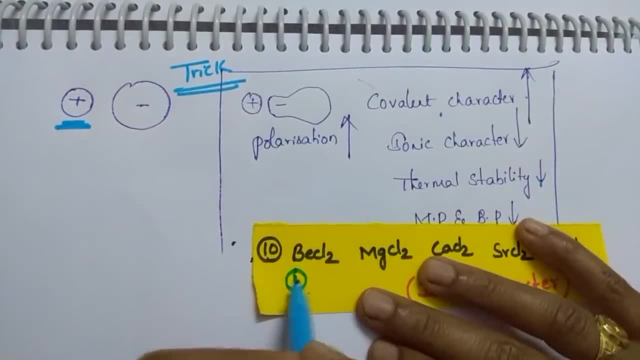 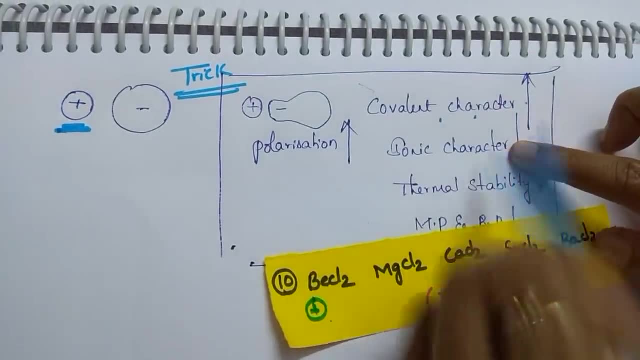 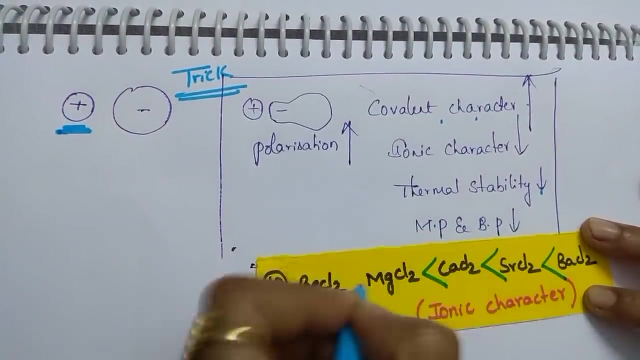 more small size of cation. here anions are same, don't worry. small size of cation. covalent character is more ionic character is less. so this is having low ionic character. then, which is having more ionic character? barium chloride, strontium chloride. this is the 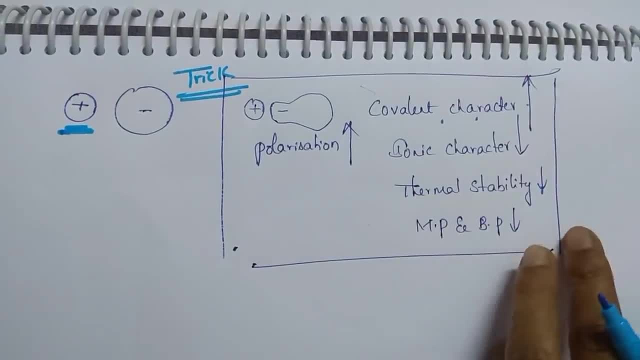 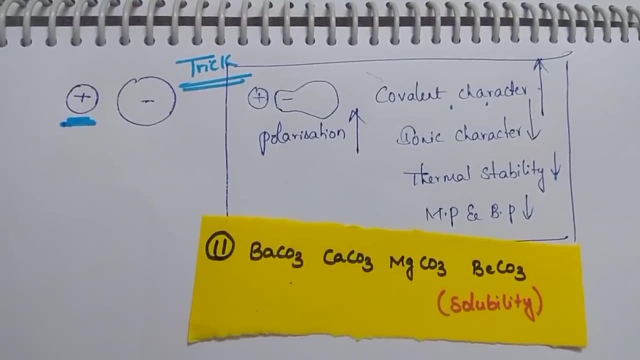 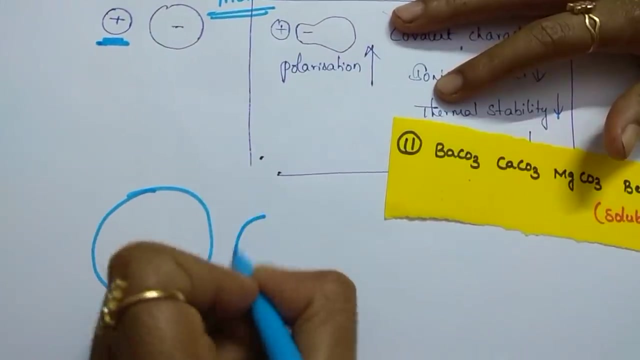 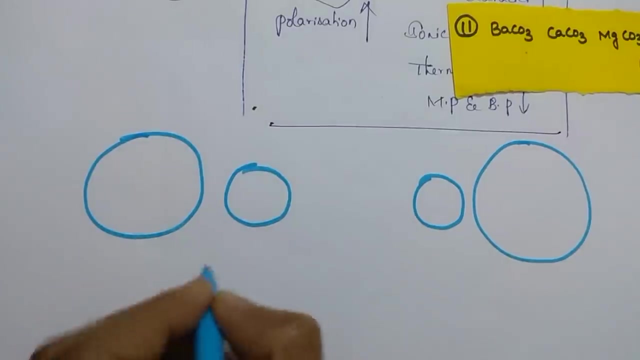 correct order, got it. next, trend solubility. Coming to the solubility, please go through based upon radius difference. here, radius difference: one cation is larger, one ion is larger, another ion is smaller. or one ion is smaller, another ion is larger whenever radius difference increases. radius difference: 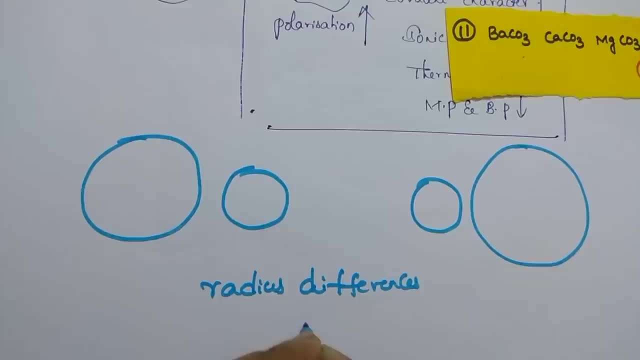 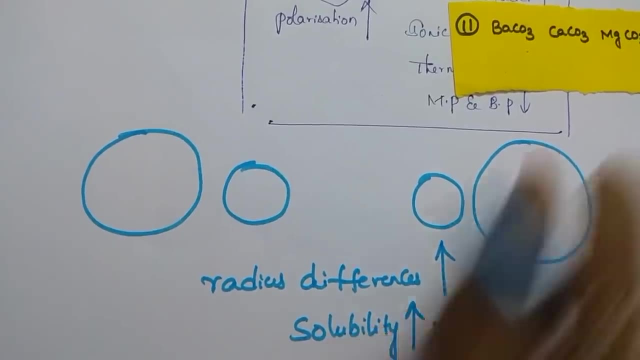 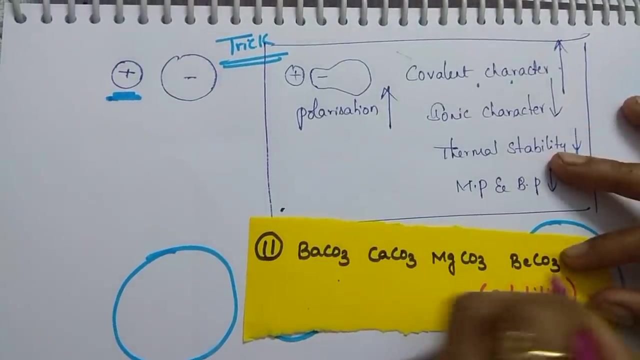 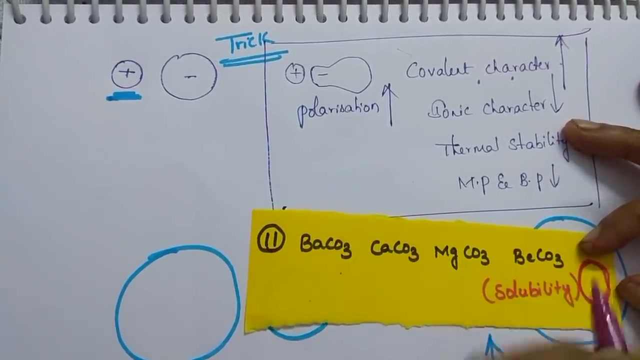 increases, then what happens is solubility also increases In this. barium carbonate, calcium carbonate, magnesium carbonate, beryllium carbonate. carbonates are same, okay, and actually carbonate ion is a larger ion, it is a carbonate one. 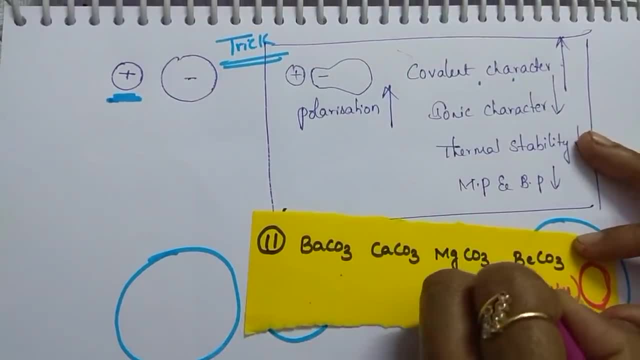 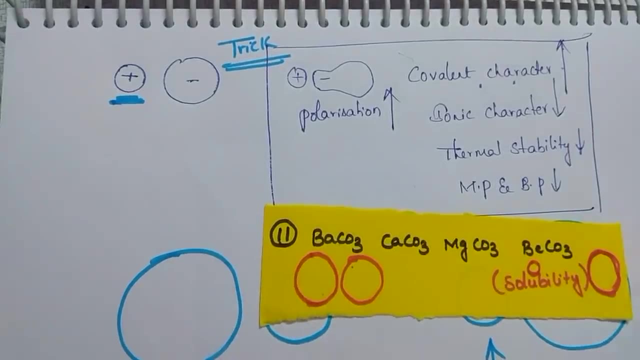 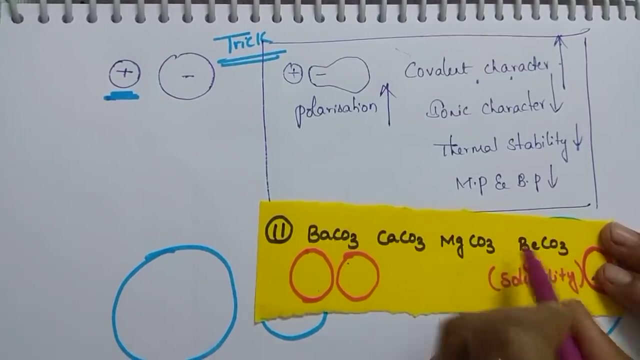 carbon, three oxygens larger ion and beryllium is a smaller. in this case, carbonate is larger. ma'am how we will come to know whether carbonate is larger? just check that more atoms is there. take it as larger anion. now this is smaller. this is a larger beryllium, smaller carbonate. 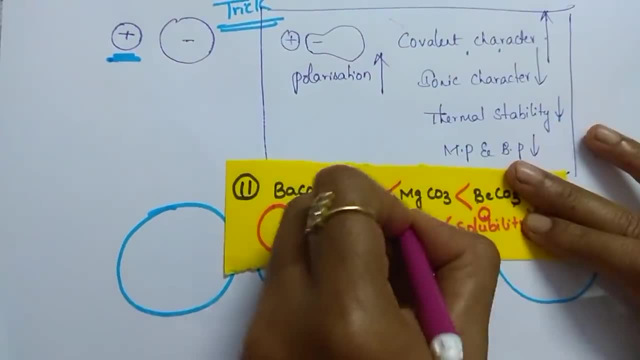 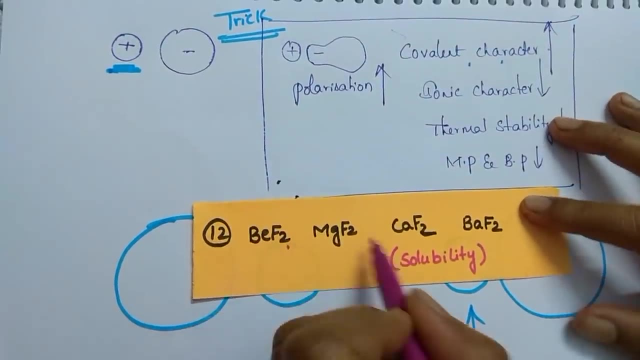 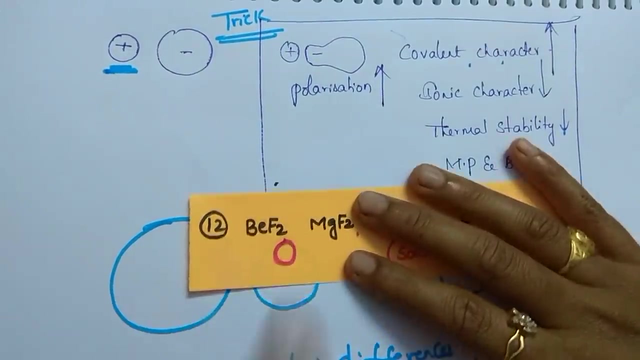 larger, so more radius difference, more solubility, clear students, easy, easy, very easy. beryllium fluoride, magnesium fluoride, calcium fluoride, barium fluoride fluoride. ion F minus is a smaller anion, so this is smaller means cation should be larger in this case. which? 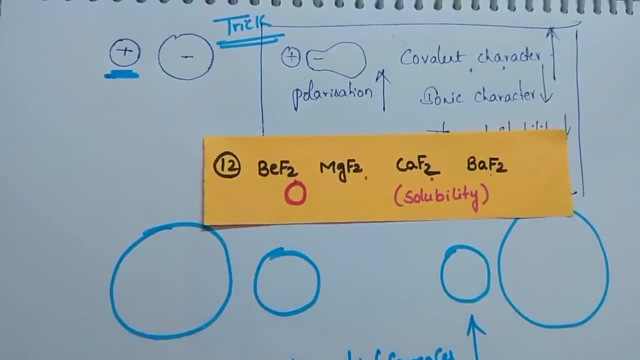 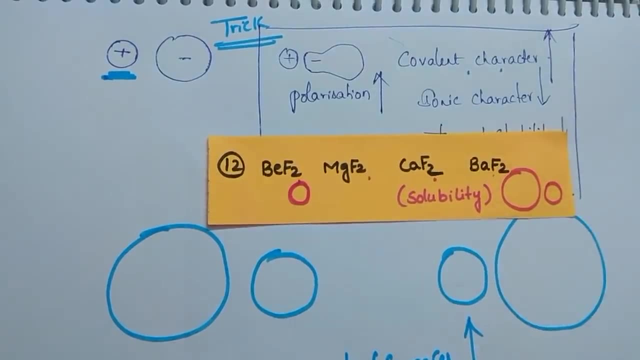 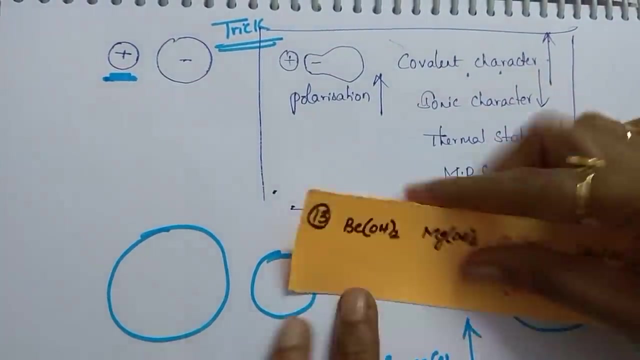 cation is larger. Beryllium, magnesium, calcium, beryllium, top to bottom. what happens? Size increases, so beryllium is larger size. fluoride ion: smaller size, so radius difference is more and solubility is more. beryllium hydroxide, magnesium hydroxide, calcium hydroxide. 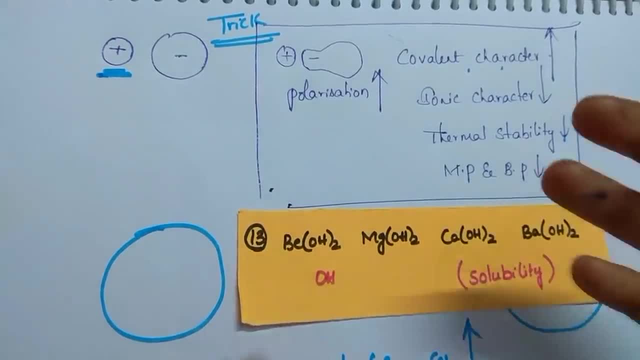 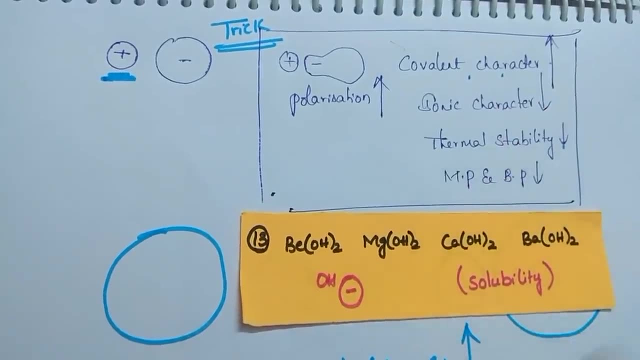 beryllium hydroxide, OH minus. consider as only two ions. consider as a smaller ion, so that oxygen and hydrogen smaller anion, so which Other other one should be? this is smaller means other one should be larger in this. 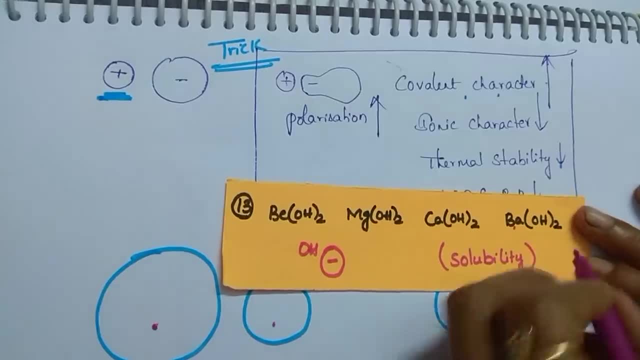 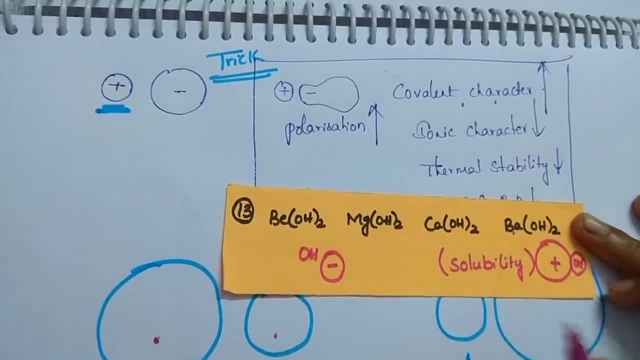 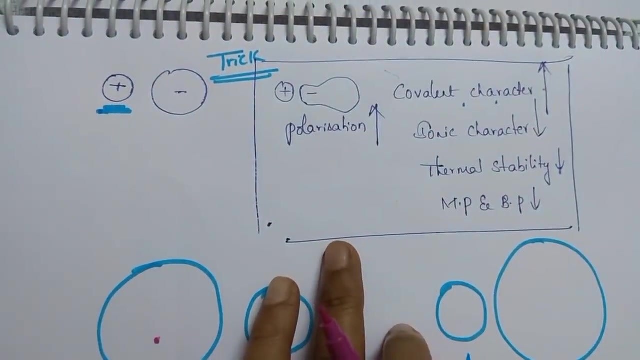 case, which is which one is a larger. Beryllium ion is larger, so beryllium ion is larger and OH minus ions are smaller, so that it is having more solubility. tell me the basic character beryllium hydroxide. 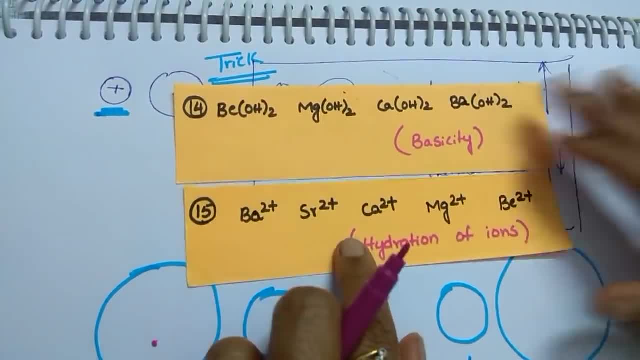 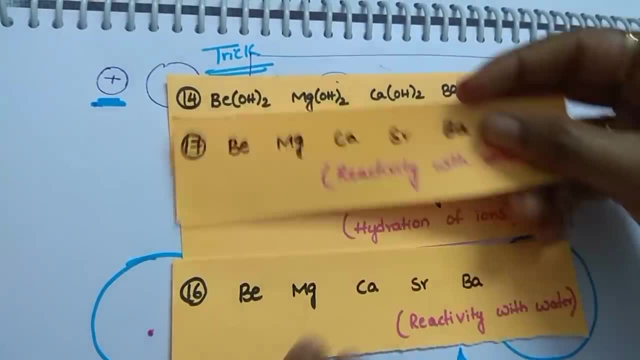 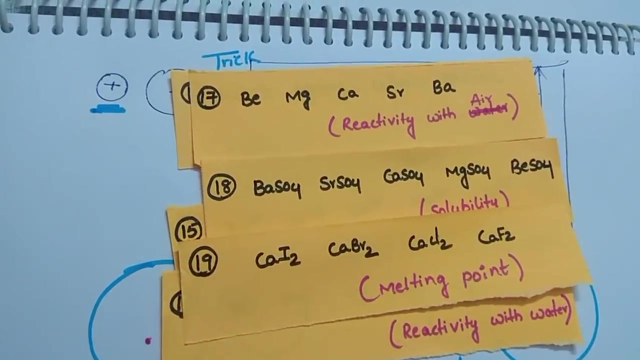 this is the next question. 14th question: Try these questions. ok, I will give you the solution in next video. copy these questions: 17th, 18th question, 19th: do it please. don't think that I understood everything.